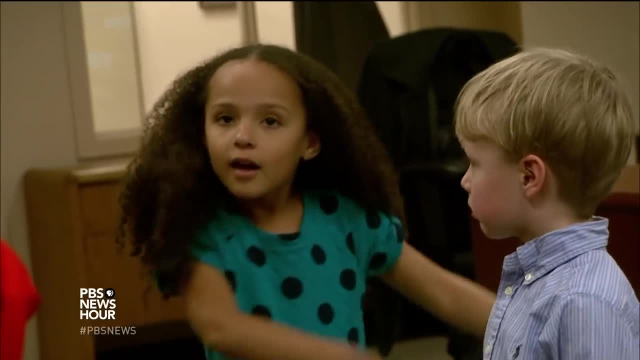 PAUL SOLMAN. What does a bank do, BETH KOBLINER? A bank gives you money and stuff, PAUL SOLMAN. They just hand it out, BETH KOBLINER? I don't think so. PAUL SOLMAN No. 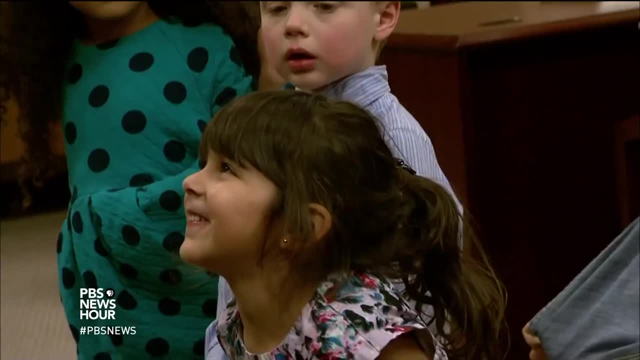 PAUL SOLMAN. Where does a bank get money? BETH KOBLINER, I think it gets from a sock. PAUL SOLMAN, From a sock PAUL SOLMAN. Personal finance guru Beth Kobliner thinks kids should be learning about. 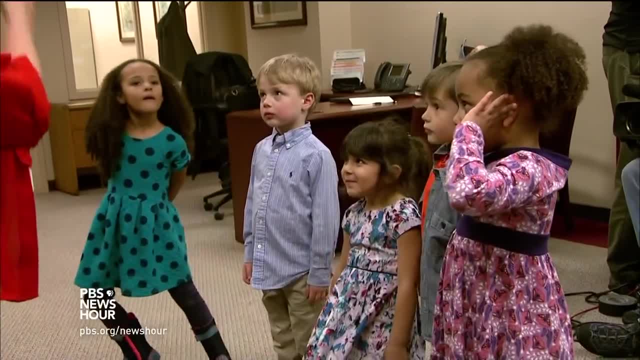 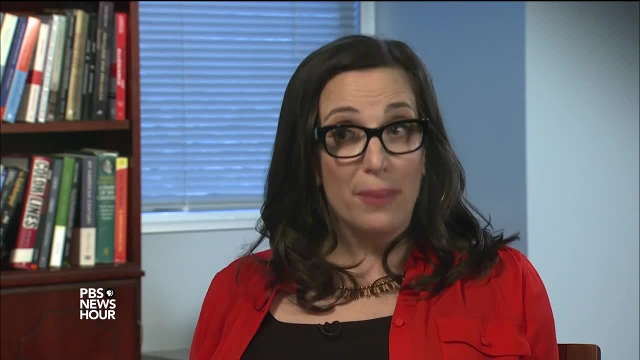 money early, but they're not BETH KOBLINER. I think parents are much more likely to talk BETH KOBLINER About sex or drugs or alcohol with their children than they are about money. PAUL SOLMAN Kobliner hopes to break the taboo with a new book: Make Your Kid a Money. 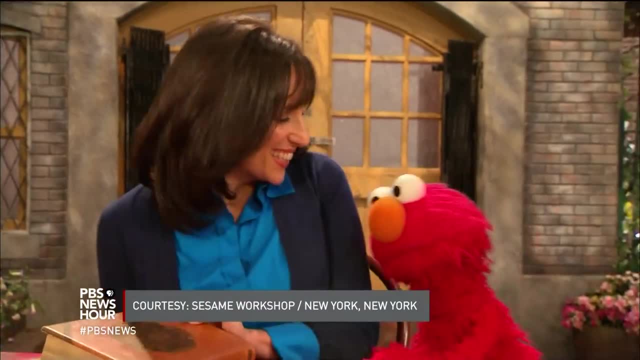 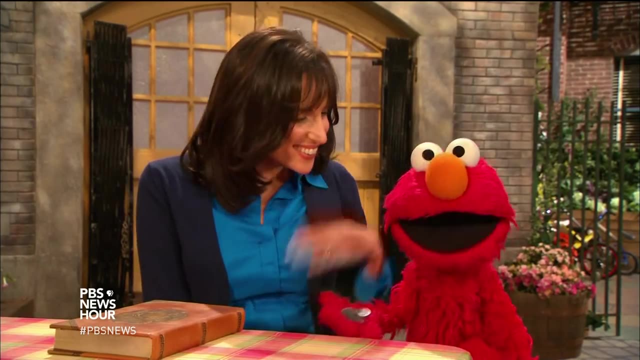 Genius that continues work she's been doing for years. Hi, Elmo. Oh, look what Elmo has. PAUL SOLMAN Kobliner has been teaching key concepts in economics. She insists kids can learn them young. What should Elmo do with all this money? 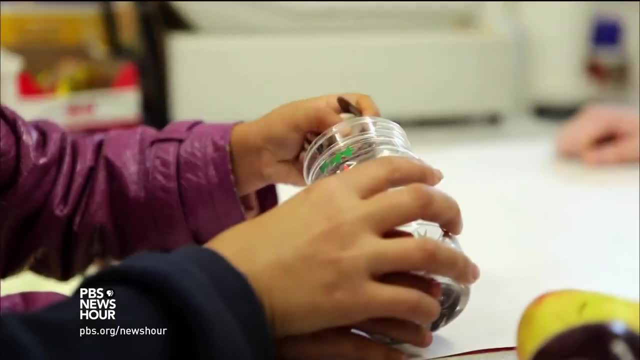 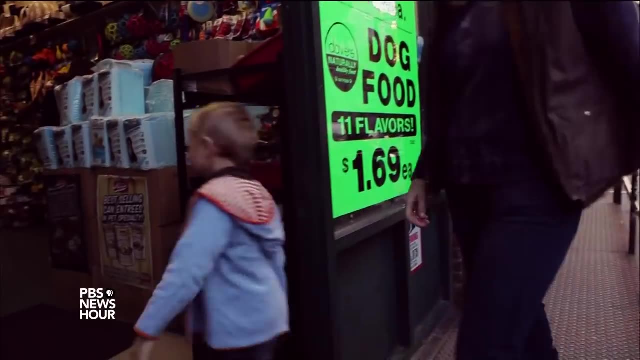 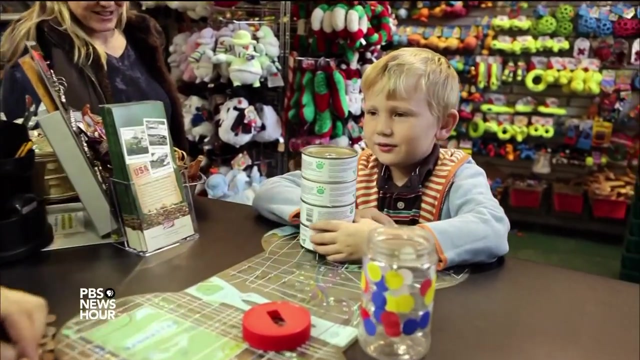 BETH KOBLINER. By age 3, children can understand basic money concepts like exchange, Or we have to make choices Or things have value, And those conversations are important to start when kids are really little. By age 7, a lot of those behaviors having to do with money, whether it's self-control, 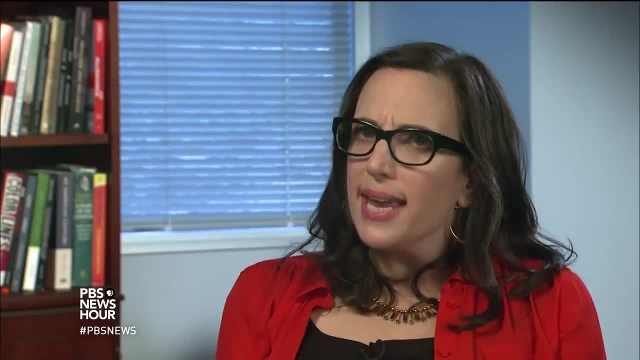 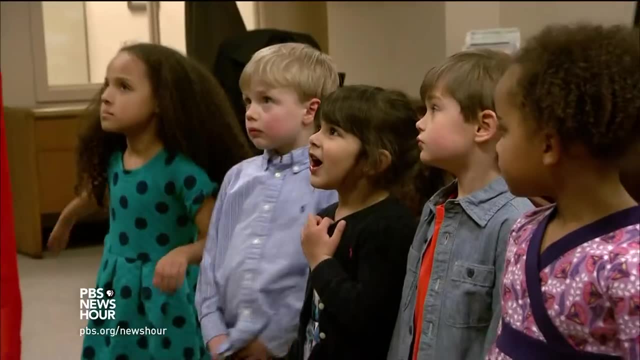 or delayed gratification they start getting set. So those ages 3 to 7 is really kind of a nice sweet spot in which parents should be talking to their kids about money. PAUL SOLMAN, We gathered our own group of kids to try it out. 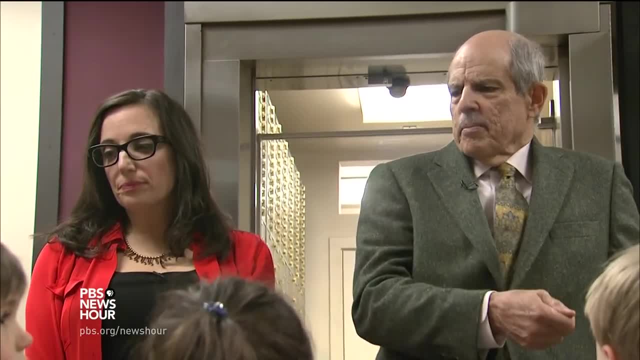 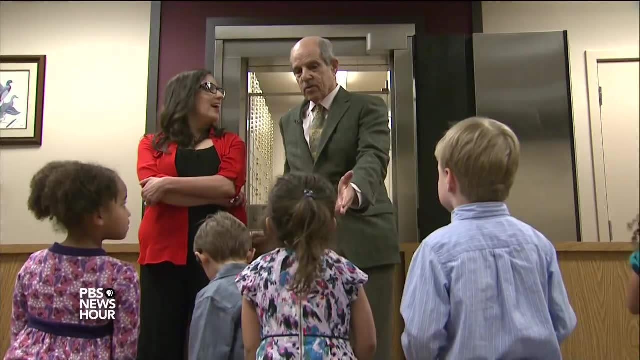 How do people get money? How do they get money? How do they get money to give to the bank? My mom and dad work and get money and they buy milk for me. PAUL SOLMAN, There you go, And you're how old here. 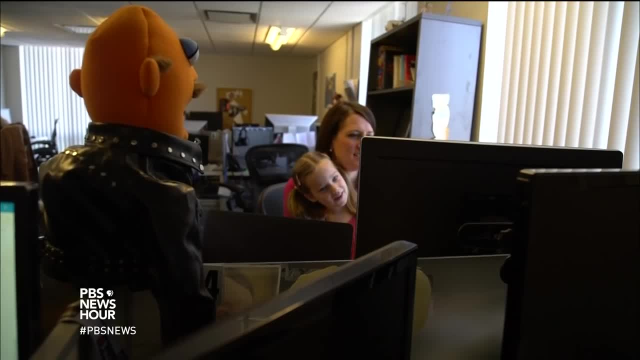 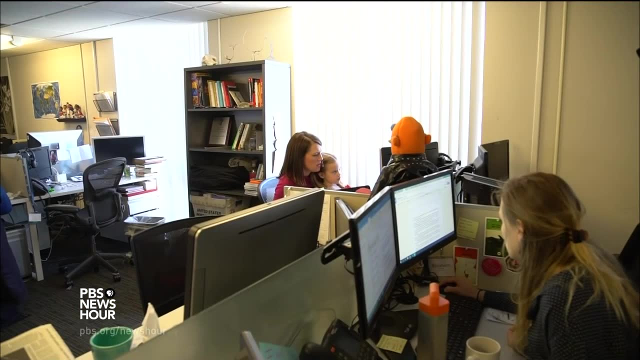 Just 3 years old. Another key concept: all kids should know, says Kobliner, what it means to work for a living. like here at the NewsHour BETH KOBLINER. You bring your kid to your office and they see where you work. 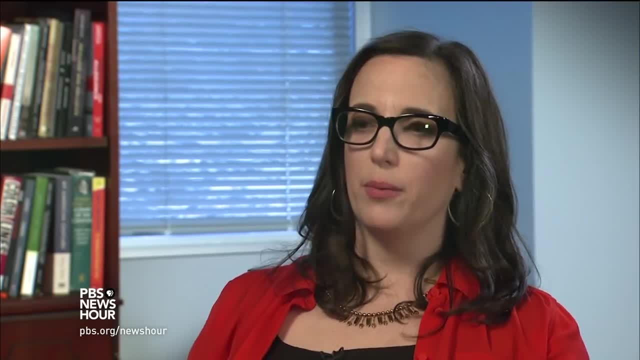 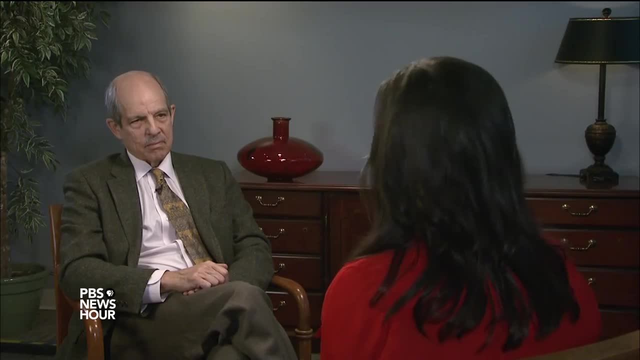 This woman I know. she said her dad would leave every morning when she was little, with a newspaper under his arm And she thought: oh, my dad's job is reading the newspaper every day. And then, years later she found out: oh, he's a teacher. 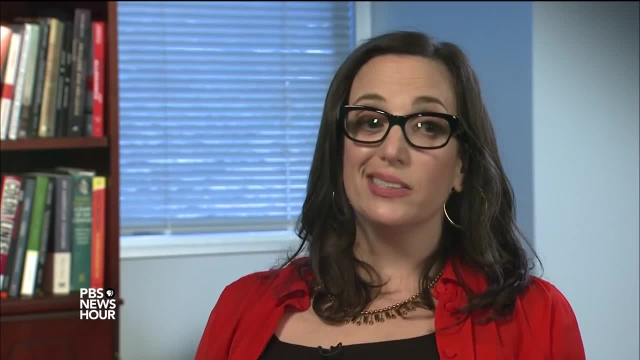 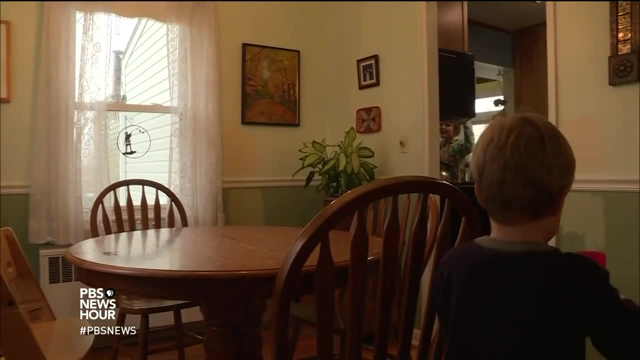 Parents say: you know how hard I work to make money for you, And kids are like: oh, I guess so. PAUL SOLMAN Kobliner also advises teaching kids to internalize the non-material payoffs from work by having them do some. 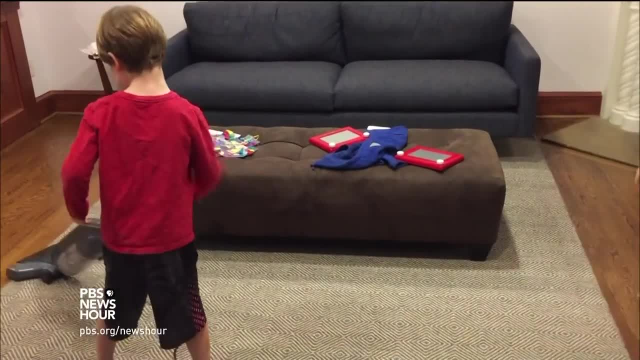 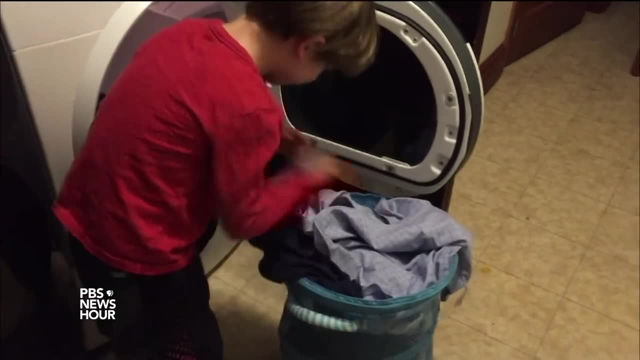 BETH KOBLINER. Having a child do chores at a really young age, and we're talking about household chores: Putting your dishes in the sink, Putting them in the dishwasher, Putting your clothes in the hamper. That type of thing at early ages- 3,, 4,, 5 years old- was one predictor of success in life. 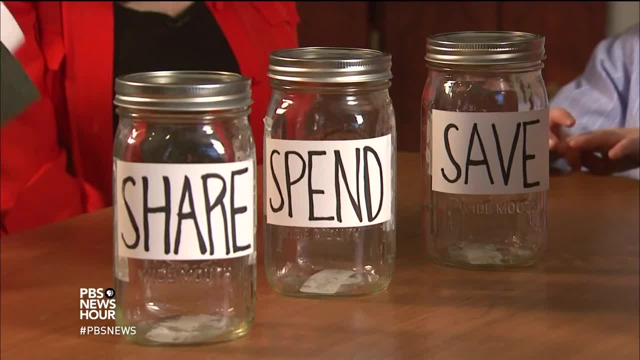 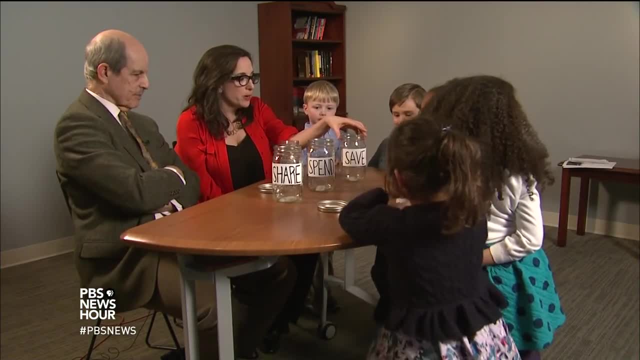 PAUL SOLMAN. Like getting a degree or starting a career, Kobliner also touts a trendy gimmick for teaching kids the uses of money: BETH KOBLINER. There are three different jars here. One is for Spending. 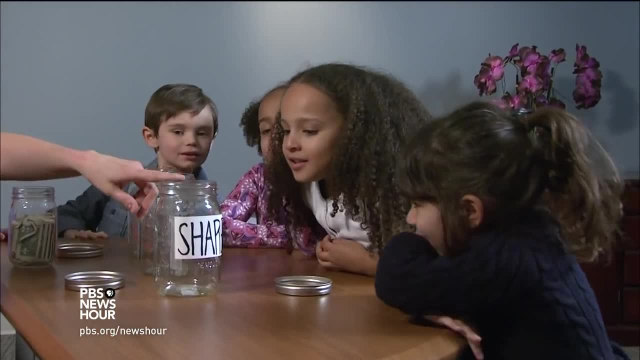 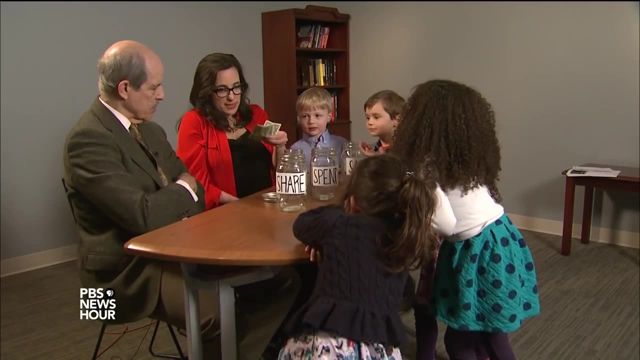 BETH KOBLINER. This one is for Spending BETH KOBLINER And this one is for Sharing Spending. PAUL SOLMAN. The key concept here: opportunity cost. If you spend, you don't have the opportunity to save or share. 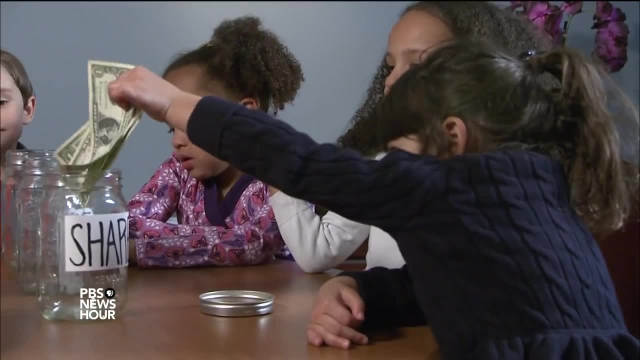 BETH KOBLINER. Which do you want to do? Do you want to save it? Share BETH KOBLINER. You want to share it? What would you do? You can either save it. Oh my gosh. 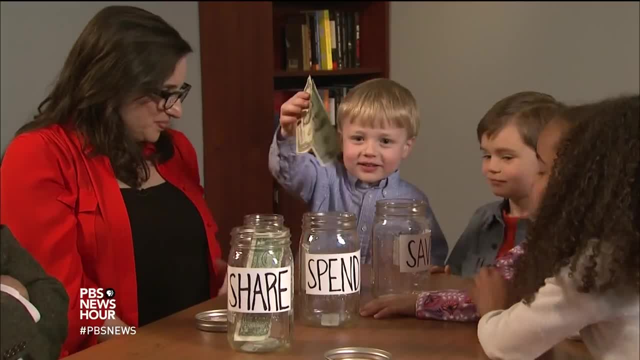 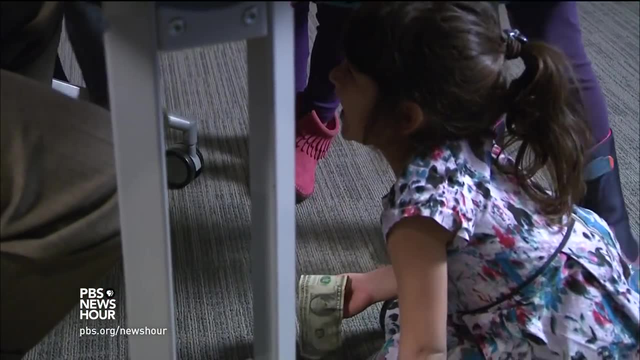 I know which one. BETH KOBLINER Which one? Tell me I'm under the table. BETH KOBLINER Spend. Where are you, Vera? I'm under the table. PAUL SOLMAN. Those of you who ducked out of econ lectures in school might sympathize. 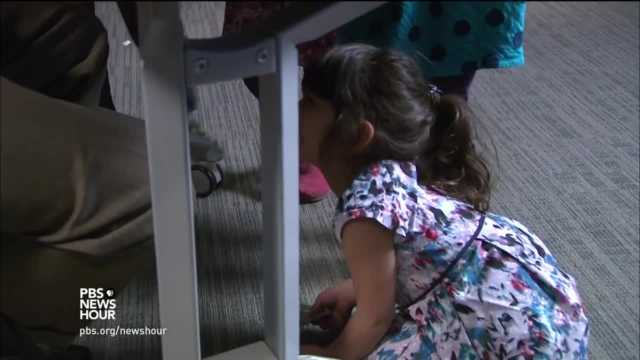 with Vera's time. It's a time-out moment, but the professor unfazed pushknot. So why do you want to spend it? What would you spend it on? Minecraft toys. BETH KOBLINER. Minecraft toys. 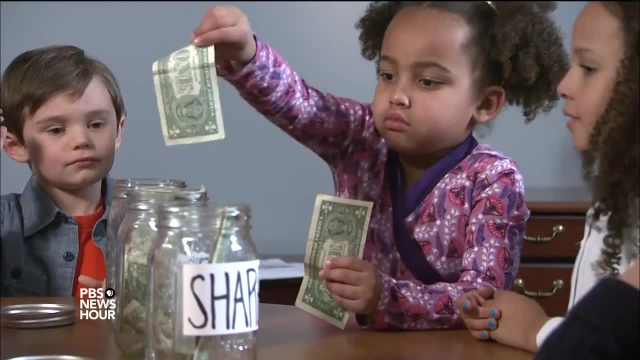 Oh interesting. PAUL SOLMAN, Whitley Wilkes, decided to put $1 in each of the jars BETH KOBLINER. That's very interesting. Why did you do that? Because I want to do all three in here. 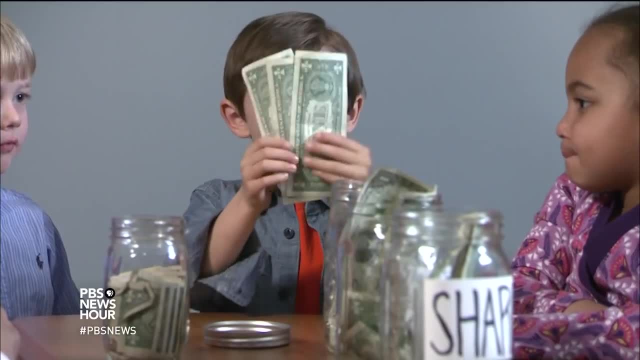 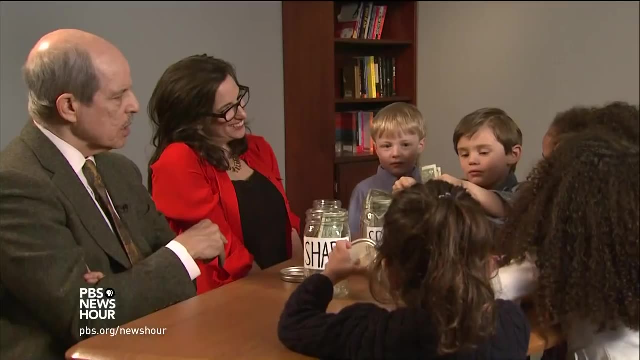 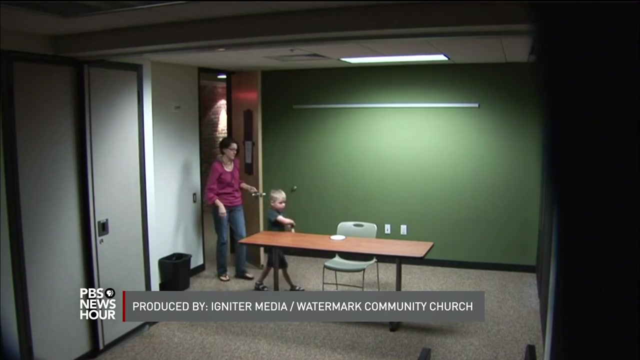 BETH KOBLINER In saving. Wow, PAUL SOLMAN, And what are you saving for Clothes, Clothes, Clothes. in high school, BETH KOBLINER? Teaching kids to save, Giving kids to save, says Kobliner is just teaching them to wait, as in the famous marshmallow. 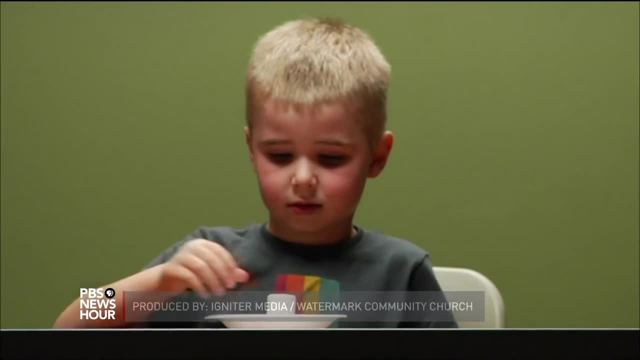 experiment: BETH KOBLINER. All right, here's the deal: Marshmallow for you. You can either wait and I will give you another one if you wait. So you can either eat it right now or you can wait. 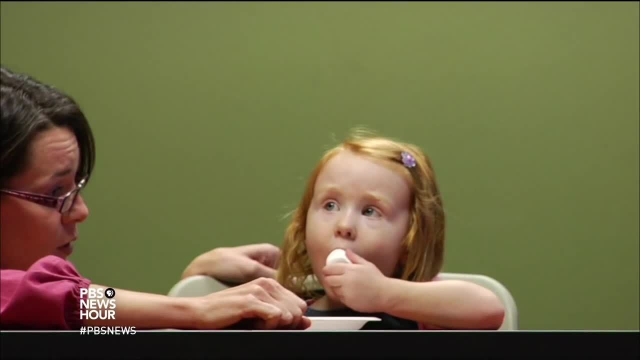 Either way, PAUL SOLMAN. We ran our own mental version. Suppose I had a marshmallow in front of you now and I said, if you don't eat it for 15 minutes, you would eat it right away, Even though I would say I would give you two later. 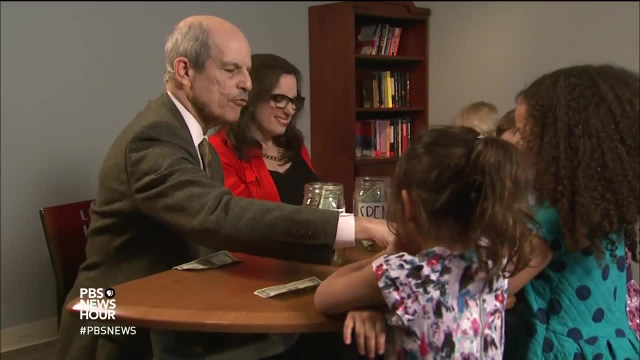 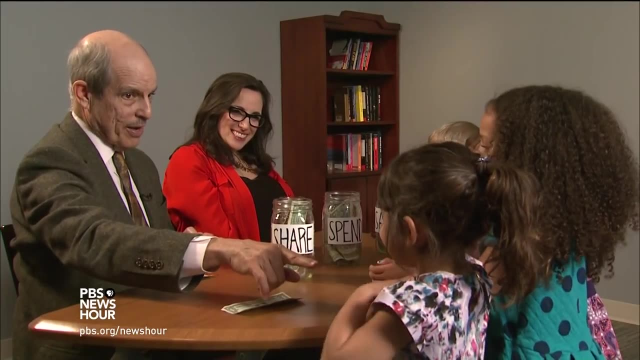 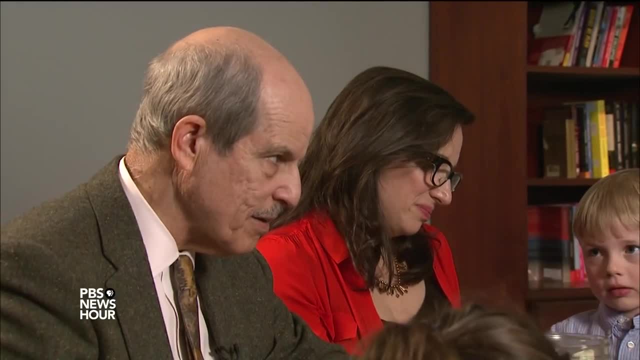 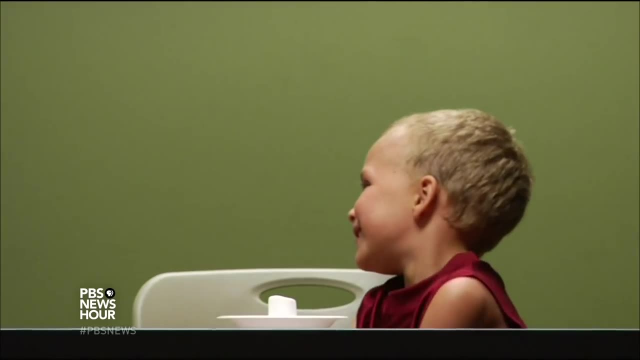 What would you do? I would wait a little while. PAUL SOLMAN, Could you wait? Yep, I would play with my Legos. If there was a fight, I would just cook it, PAUL SOLMAN. Well, no marshmallow toasting in the actual experiment. 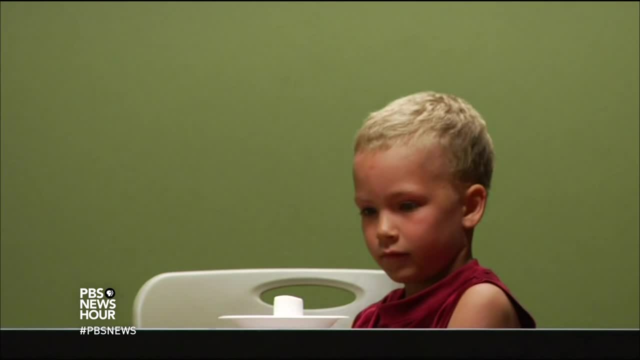 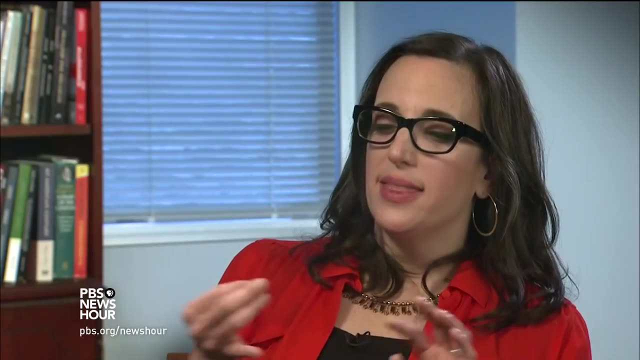 Kids were left alone in a room with a mouth-watering morsel right in front of them. In follow-up studies, those who waited longer actually fared better in life. BETH KOBLINER Teaching kids to save. They had 200 points on average higher on their SATs. 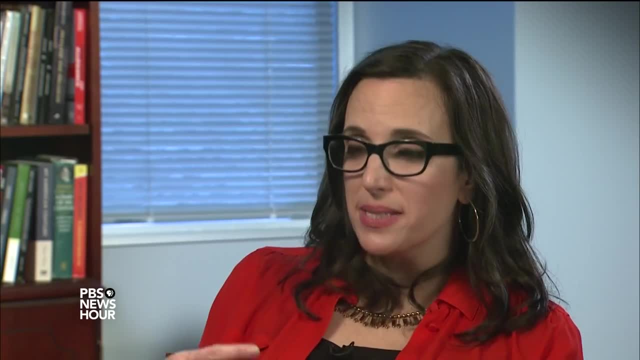 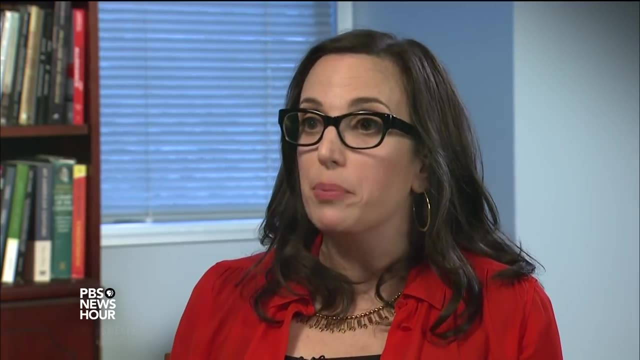 They had better interpersonal relationships And they even had lower body mass indexes. It feels at first like: oh, it's because these kids have this strong moral fiber. JEFFREY BROWN And higher IQ or something. MARGARET WARNER And higher. 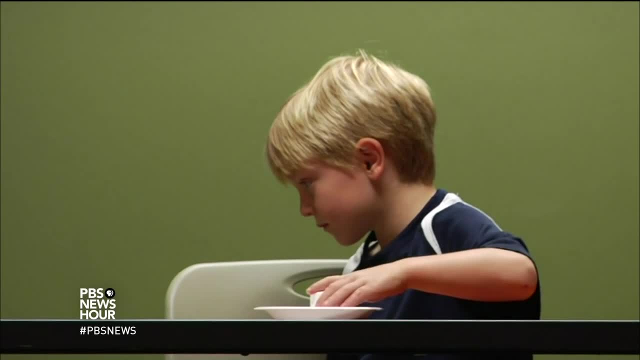 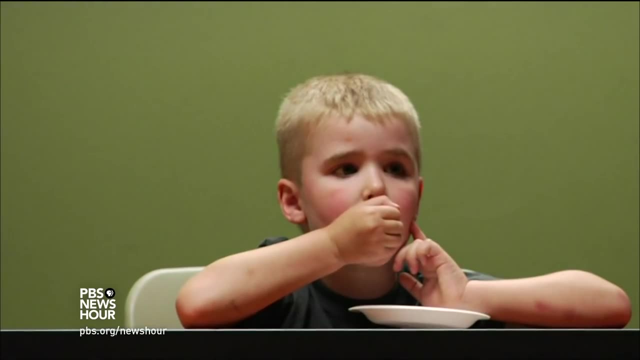 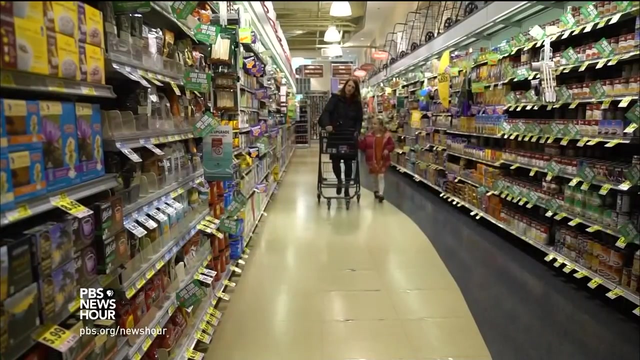 And they're able to resist it. But we also know now it's more the ability to distract themselves. That's an important trait to have. People who are able to have impulse control or delay gratification are able to save more money, JEFFREY BROWN. But how to encourage kids to delay gratification starts, says Kobliner. 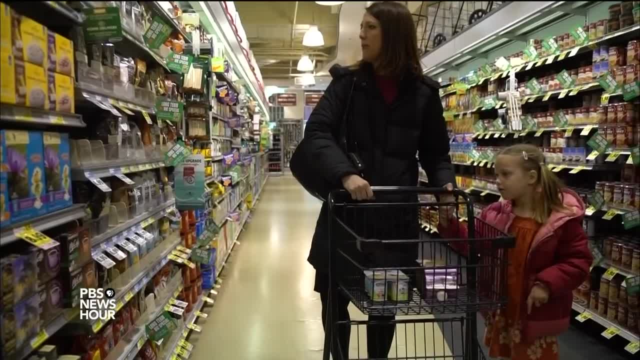 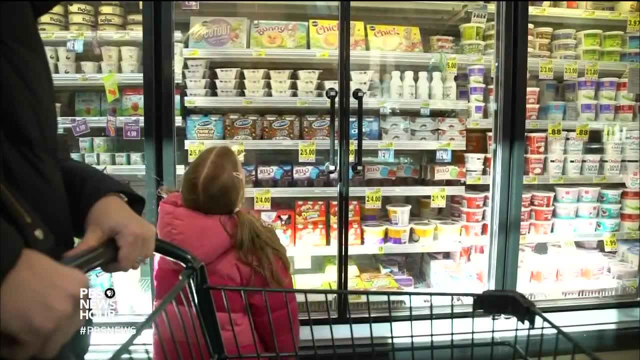 by not giving in to every demand. MARGARET WARNER, You know we're going to go into the store right now and we're only getting things we need. Research is showing when you say yes all the time, all the time, all the time you. 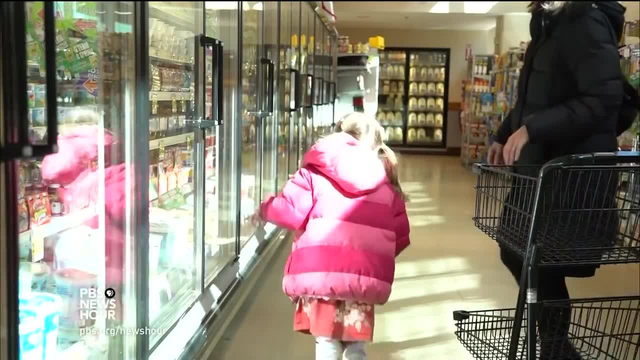 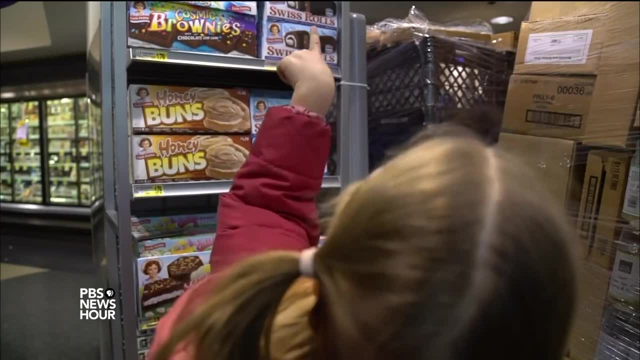 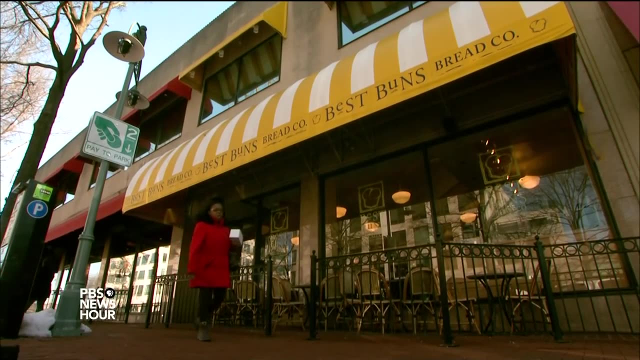 are basically, You know, making it harder for your kid to experience impulse control, Just like another study found those kids were more likely to be in debt problems because they always got what they wanted when they wanted it. JEFFREY BROWN, Beth is going to give you some real money. 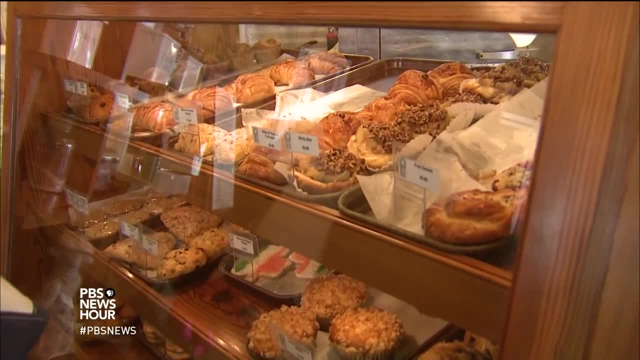 JEFFREY BROWN. Last stop, a bakery near NewsHour offices in Arlington, Virginia. Do you want to save it, share it or spend it? JEFFREY BROWN? We gave each kid $3.. What do you want to do? 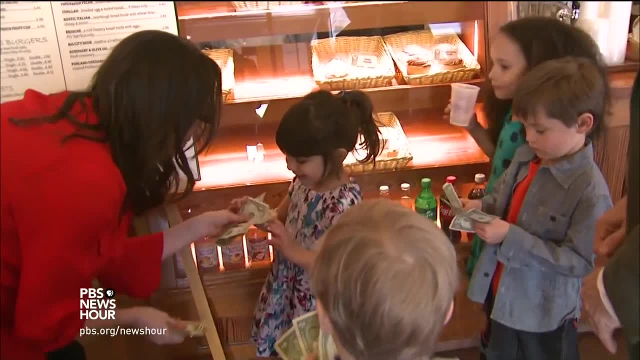 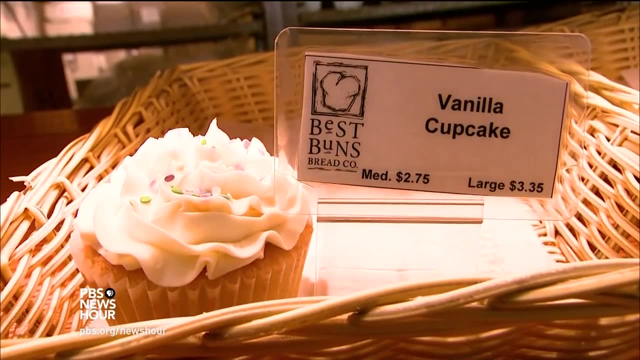 Share it. You want to share it. Who are you going to share it with? And JEFFREY BROWN. Oh, Oh, that is so sweet of you, JEFFREY BROWN. Turns out, however, that the allure of an almost $3 cupcake was 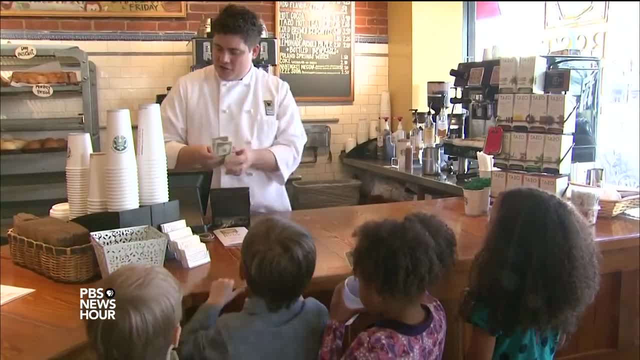 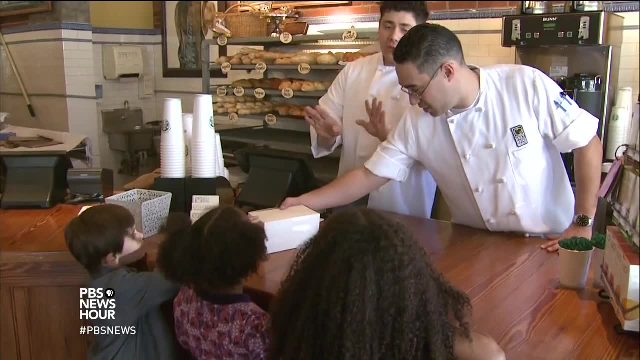 irresistible JEFFREY BROWN. Ultimately, everyone succumbed, providing Kobliner with a segue to another of her concepts, MARGARET WARNER. Is it better to buy things with a credit card or with dollar money, paper money like that? 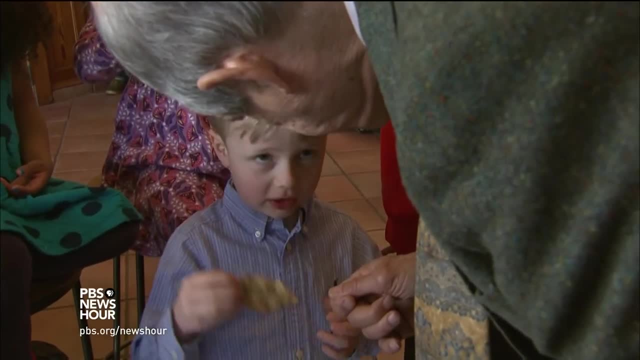 Dollar money. I would do credit cards. JEFFREY BROWN. All right Credit card, JEFFREY BROWN Credit card. Let me get off JEFFREY BROWN. You think credit card is better to? 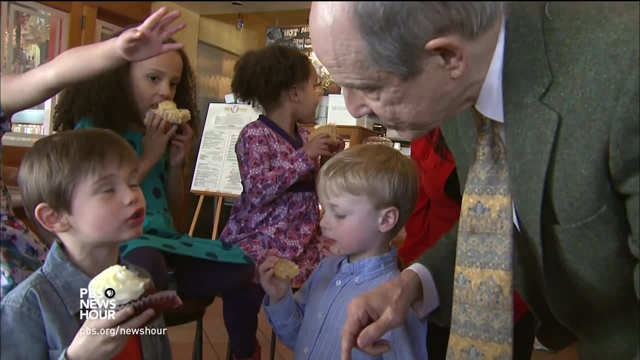 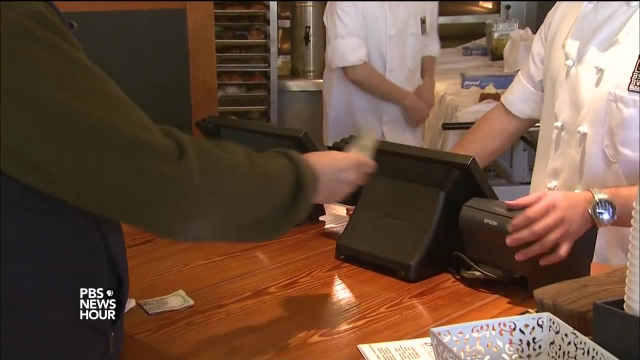 What did you think? I think it's better to use the credit card so we can save money. JEFFREY BROWN, You won't be surprised to hear that Kobliner recommends cash. so kids are aware they're actually spending when they buy something. 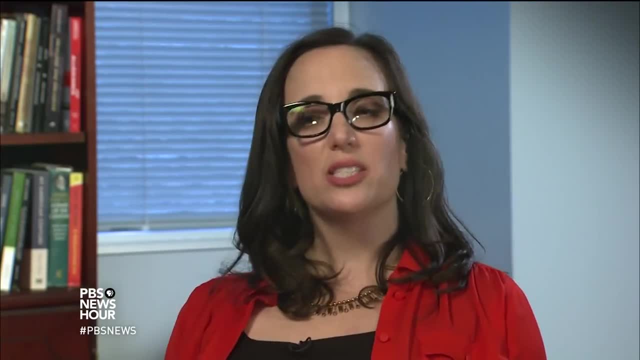 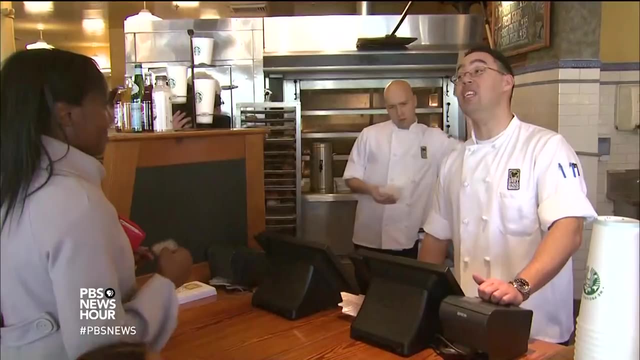 MARGARET WARNER. They don't see cash anymore. They see cards being swiped and phones now being swiped with Venmo and Apple Pay and all these ways of paying for things. JEFFREY BROWN: Yes, A recent study found that when people use a card, they spend up to twice as much than. 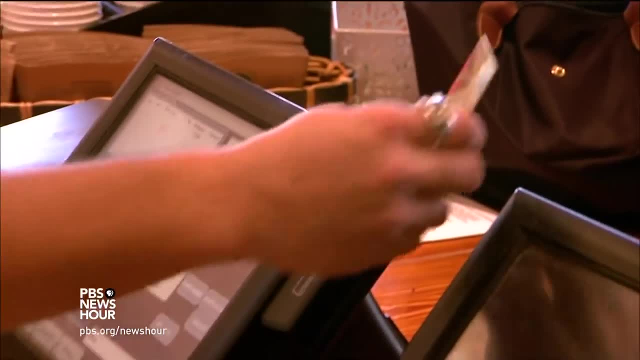 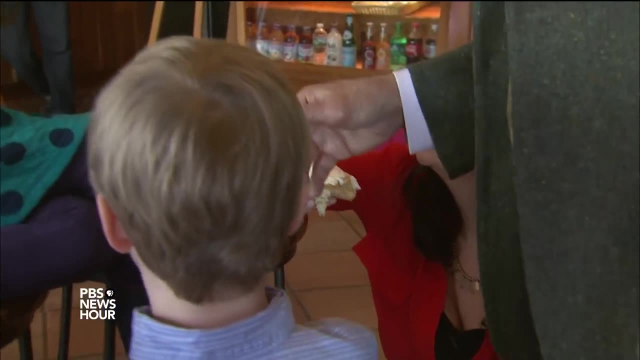 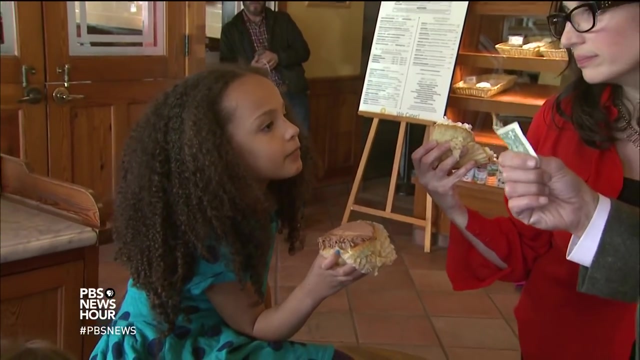 when they use cash, JEFFREY BROWN. As for paying off credit cards to avoid interest, OK, hold that till middle school. Of course, Kobliner acknowledges that teaching econ to tots isn't always easy. Why do you now think it's better to buy with cash than a credit card? 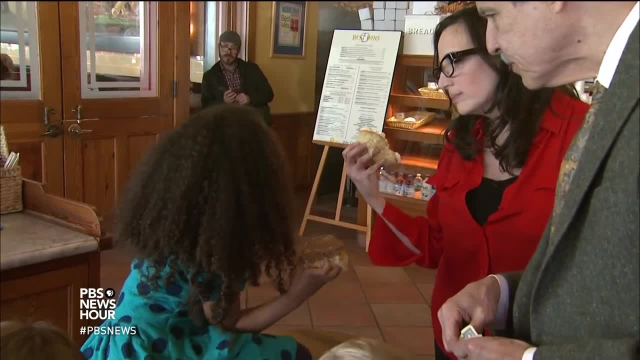 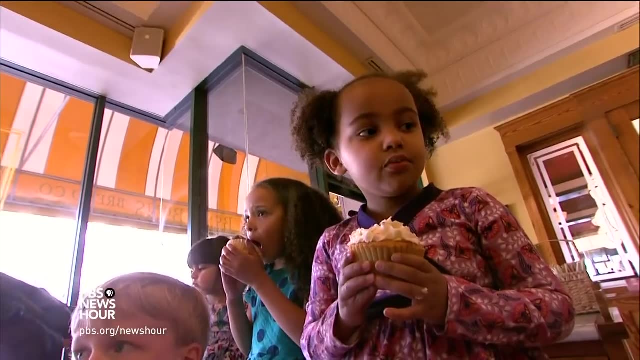 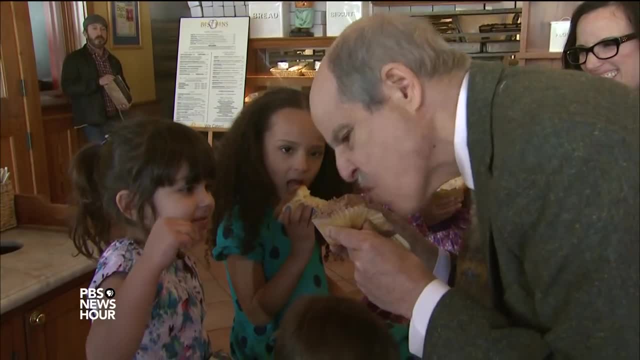 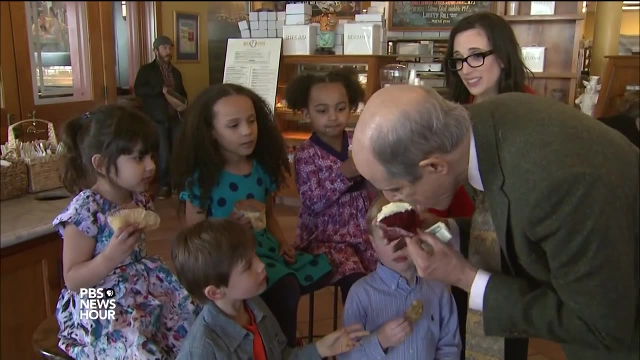 Sometimes the results can be simply delicious. This is economics correspondent Paul Solman, PAUL SOLMAN, And he is reporting from Best Buns Bakery. PAUL SOLMAN, Thank you so much. JEFFREY BROWN, Thank you. 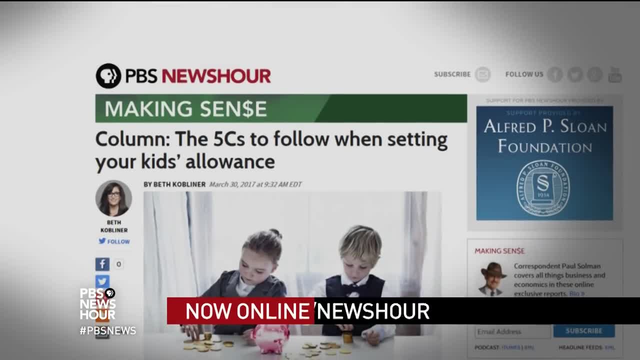 PAUL SOLMAN. Thank you, JEFFREY BROWN. Thank you, PAUL SOLMAN. Thank you, JEFFREY BROWN. Thank you, PAUL SOLMAN. Thank you, JEFFREY BROWN. Thank you.